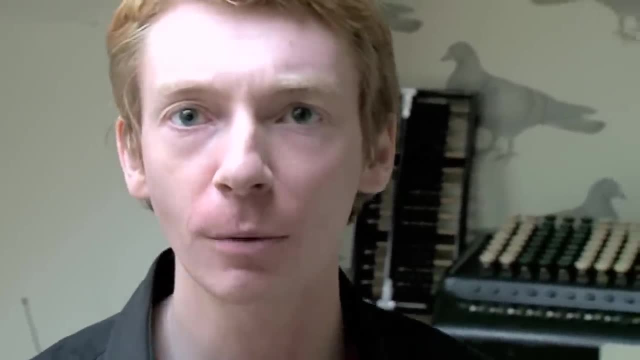 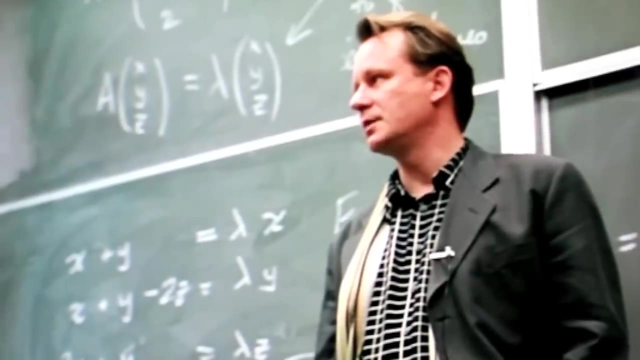 And the maths is less important. Shall we talk about what they did in the film the maths? Yeah, All right, so we'll talk about that first. Near the beginning of the film, the MIT professor sets his students a challenge: Who can solve this? I put it on the blackboard in the corridor. 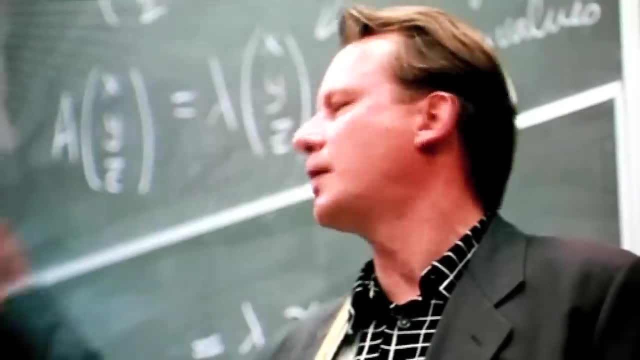 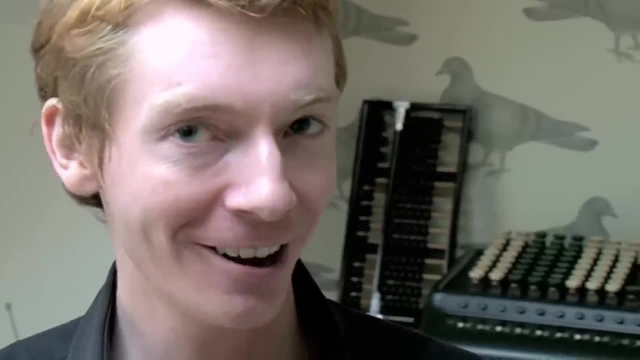 And who can solve this problem? It's taken- It's taken MIT professors- two years to solve this problem. Can you do it Now? is it as hard as he made out? So what was the problem? If I say it first of all, I'm going to say the problem that he gave the students. 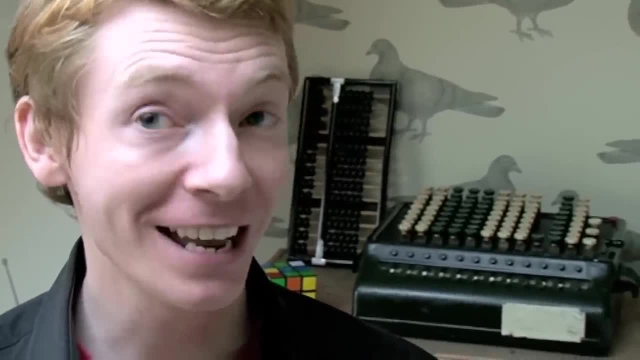 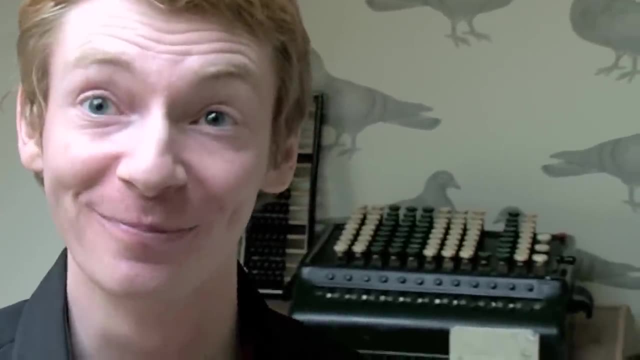 It might sound like Greek to you, because some of it is Greek, Right? So then I'll say the problem, Then I'll tell you how it works. And it's a problem we can all do at home. All right, I promise. 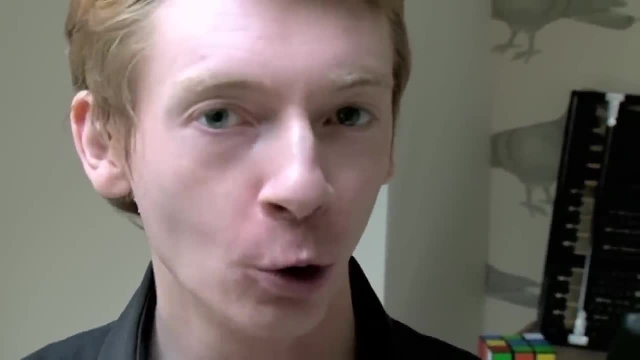 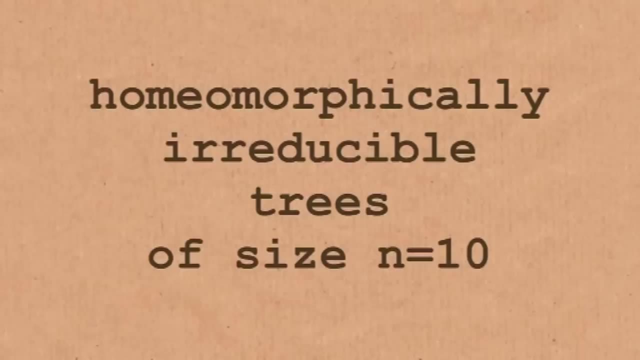 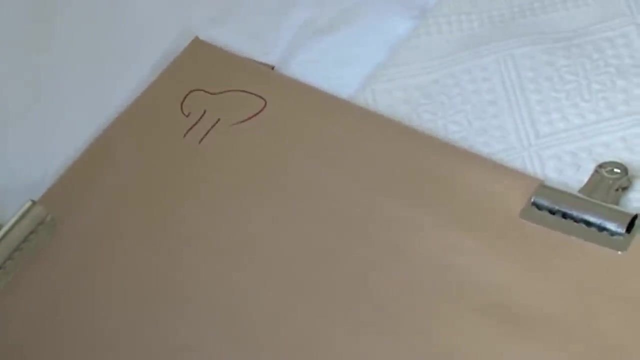 So the problem is: draw all homeomorphically irreducible trees of size n equals 10.. What does that mean? All right, let's try this out. These things are called trees, So yeah, So trees Instead of that. 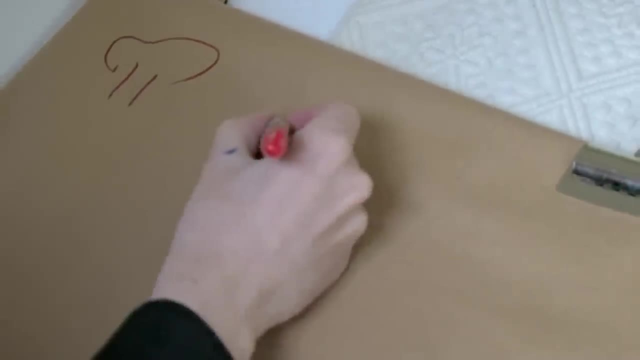 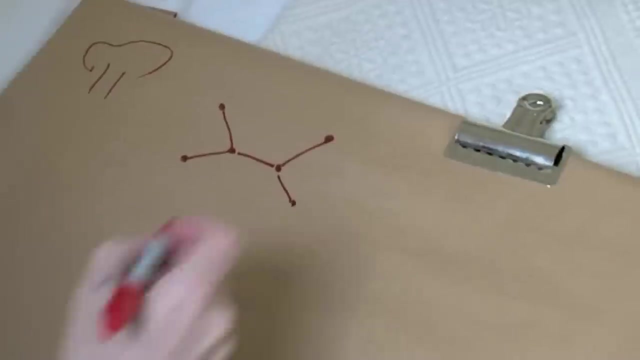 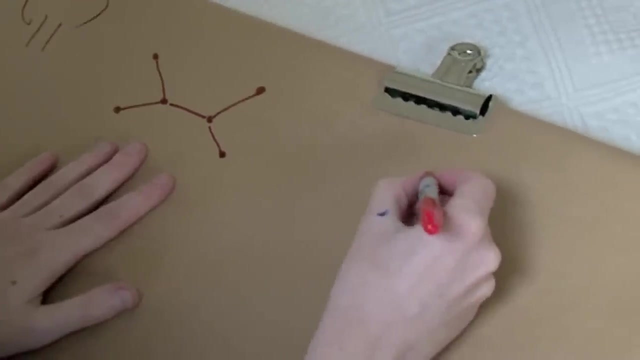 where they are networks of dots and lines, So these are called graphs. It's like the London Underground map, So a network of dots and lines. So this is called a tree. What's not allowed, what is banned, is something like this: 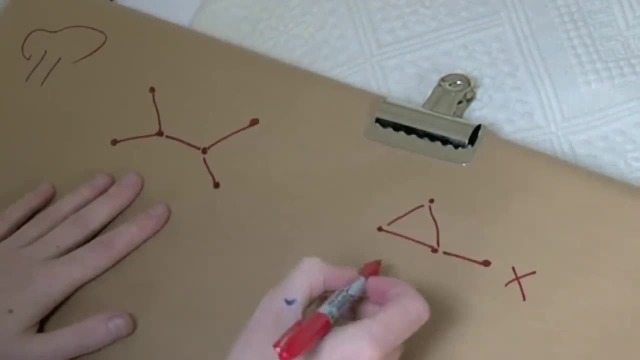 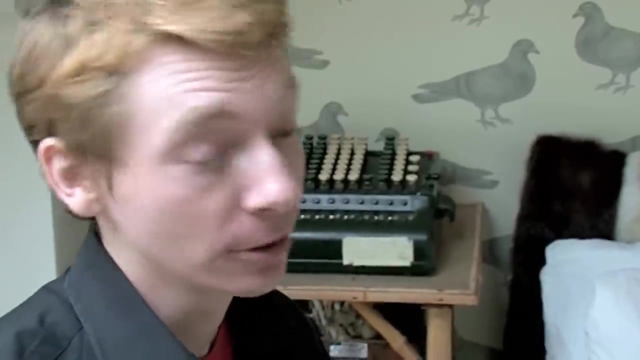 OK, This is banned. This has a cycle in it and cycles are banned. Now, what was that other big word I said Homeomorphically, That's the worst one. That's actually not so bad. That means, if I did this. 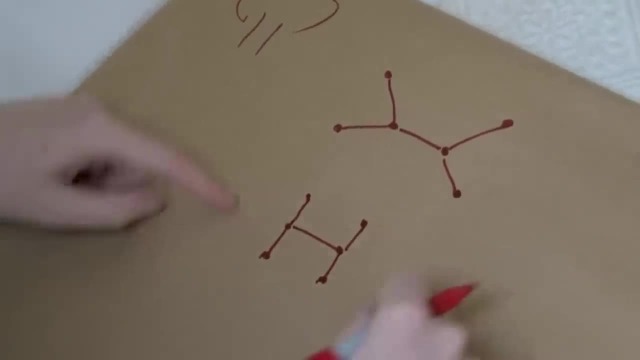 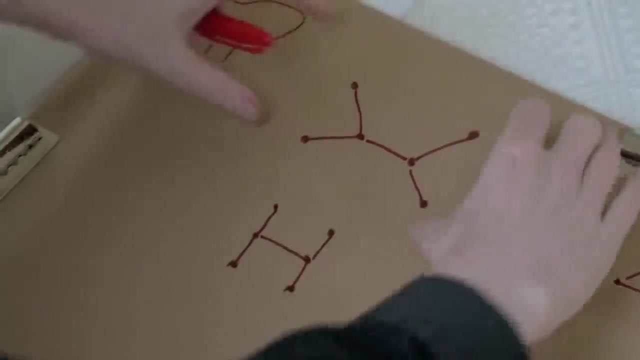 these two are the same picture. Can you see what I've done? I've just moved the dots slightly So you can rotate them and reflect them, or you could move them around slightly, But those two pictures would count as the same thing. 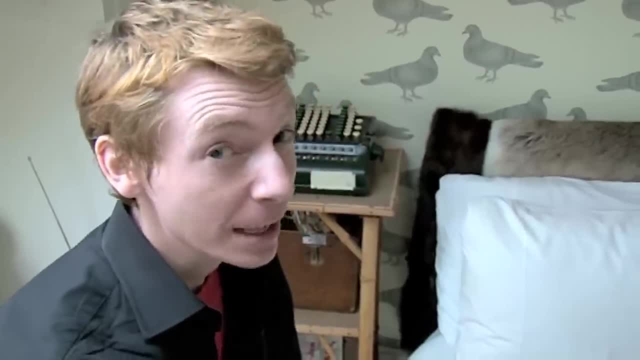 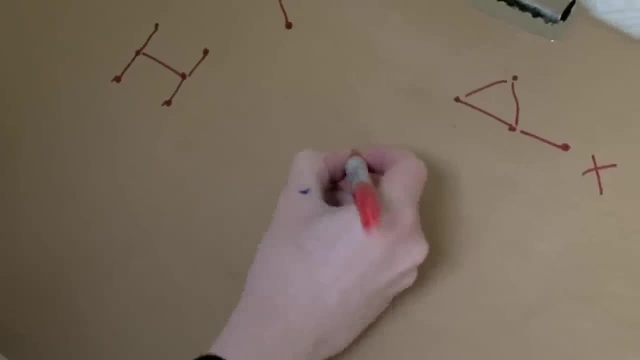 And there was another clever word. There was the word irreducible in there. So that's another banned thing here. This time what is banned is something like this: This is banned. Only two lines go into that dot, Which means pretty much nothing happens.